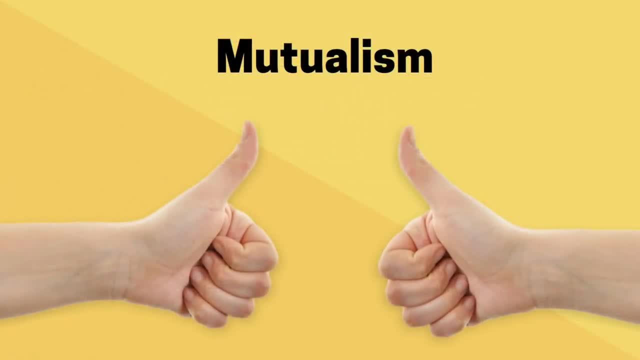 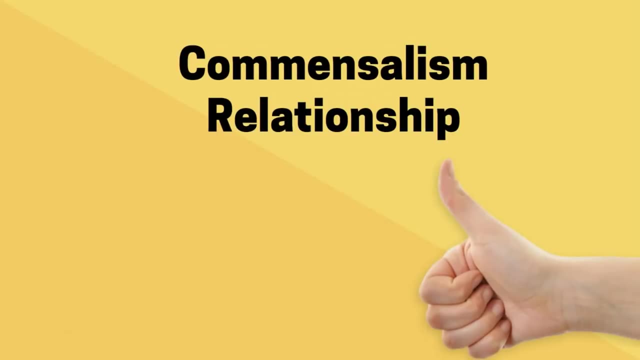 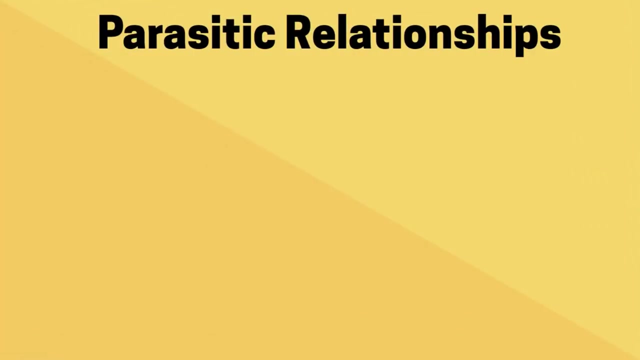 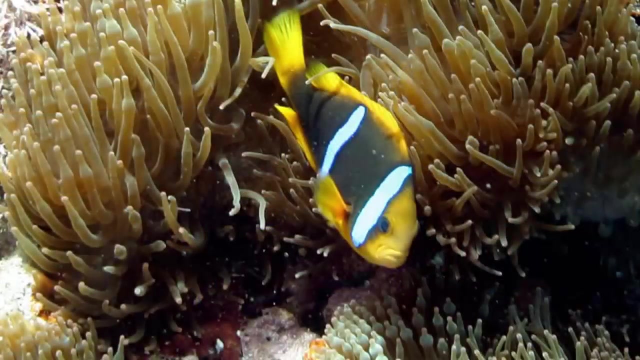 With mutualism, both organisms benefit from the relationship. With commensalism, one organism benefits and the other organism is neither harmed nor helped, Kind of like neutral. In parasitic relationships, one organism benefits while the other organism is harmed. Organisms live in very close symbiotic relationships with each other, which means one or both rely. 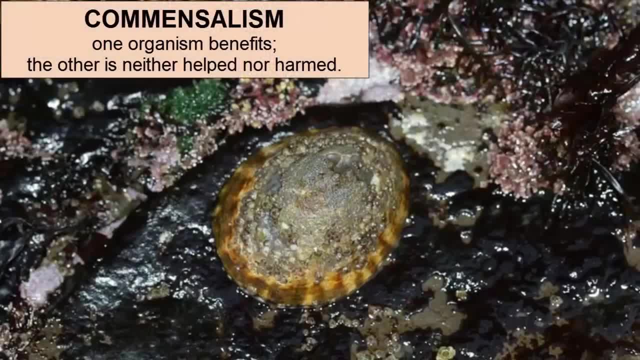 on the other for their survival. One type of symbiosis is called commensalism, in which one organism benefits and the other isn't harmed or helped. This owl limpet is being used by the tiny buckshot barnacles as a substrate on which. 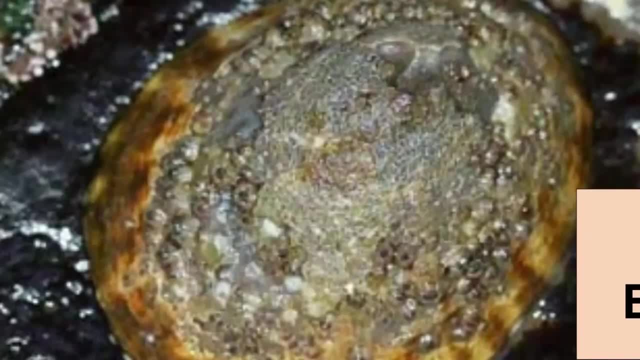 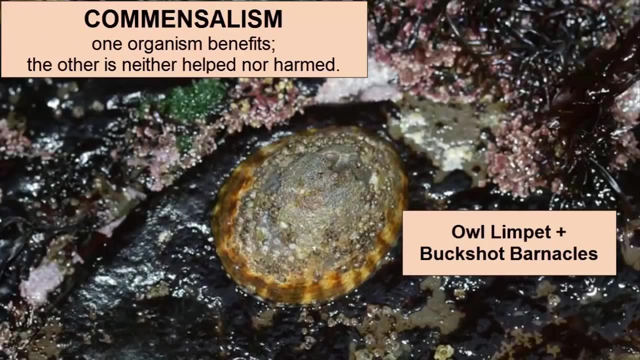 to grow. As the owl limpet moves over the rock, the barnacles are carried through the water column, giving them greater access to food. Barnacles get their food by filtering it out of the water. They remain fixed in location and so are depending on the abundance of planktonic organisms living. 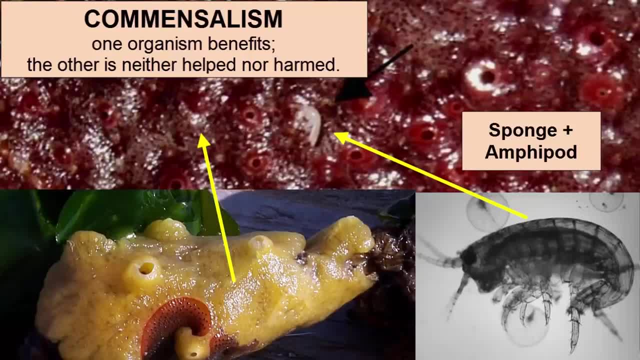 in the water around them. Another example of commensalism is shown in this picture. here This small amphipod is living attached to the outside of a sponge. Sponges filter huge quantities of water through their pores every day. This amphipod sits outside one of those holes and feeds itself off the organisms in the 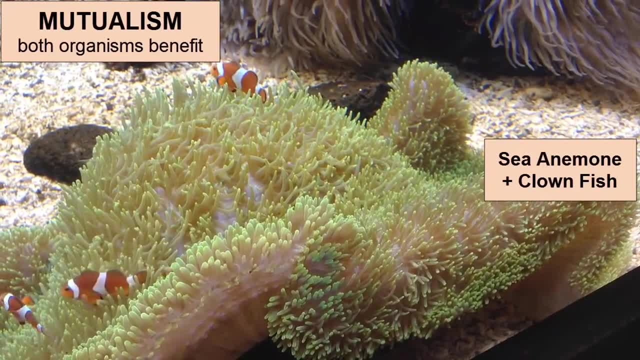 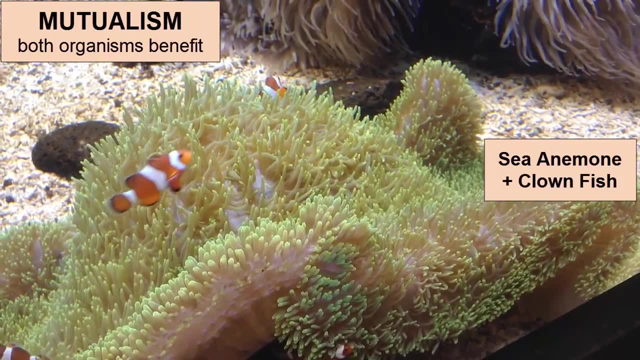 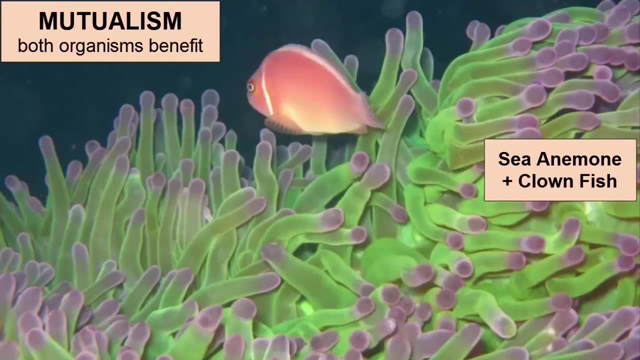 current Mutualism is a form of symbiosis in which both organisms benefit. An example is shown here with anemone and clownfish. Stinging cells in the anemones can scare off the predators of the clownfish. The clownfish has developed an immunity to the toxins in the stinging cells and they 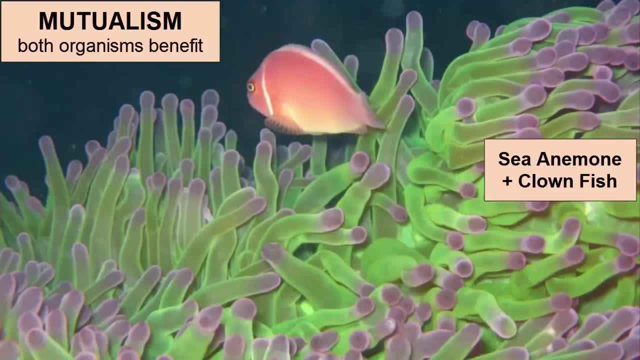 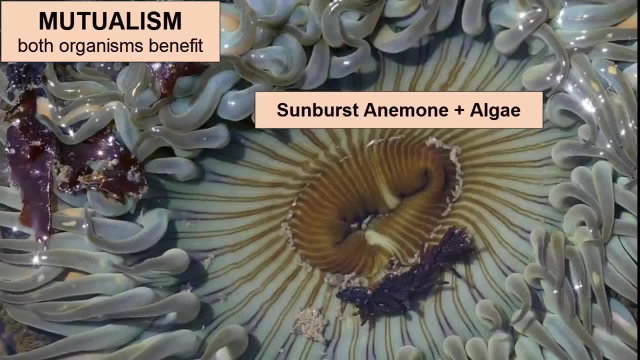 hide in the anemone, But they also can aggressively attack and scare off the anemone's main predators, sea stars and sea snails. So both benefit. Another example of mutualism happens in science: The sunburst anemone on the Pacific coast is a very common species of plant. 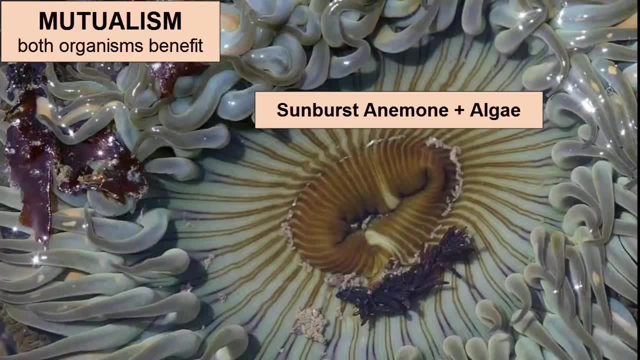 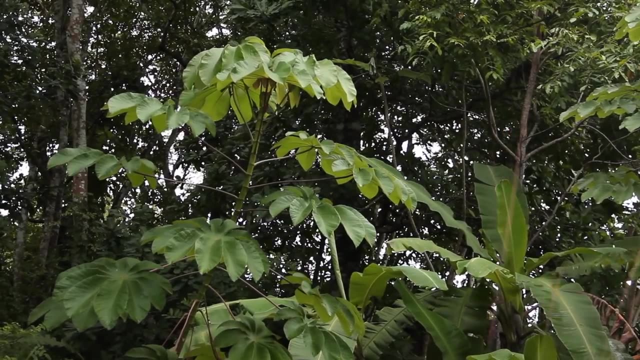 Its green color comes from tiny photosynthesizing algae that live within it and get their nutrients from the waste of the anemone. The anemone in turn feeds off the garden of algae as needed to supplement its own food source. The anemone is found in clearings and forest gaps in tropical rainforests. 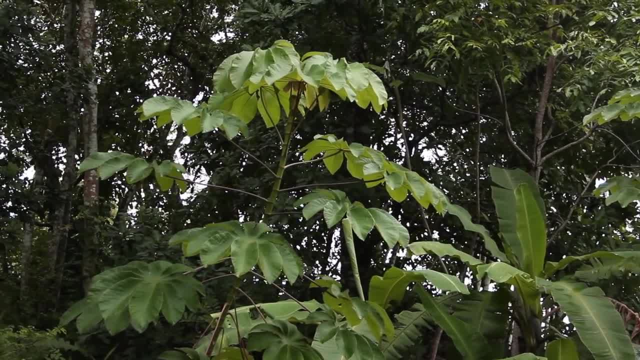 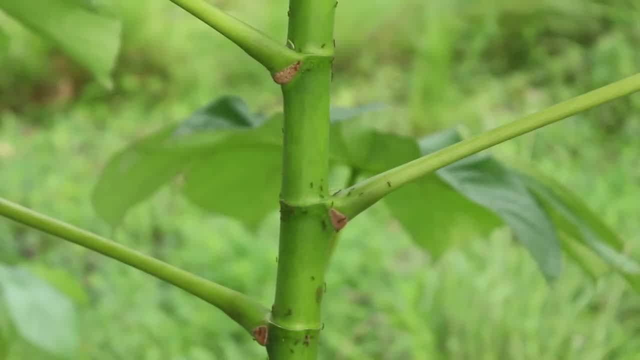 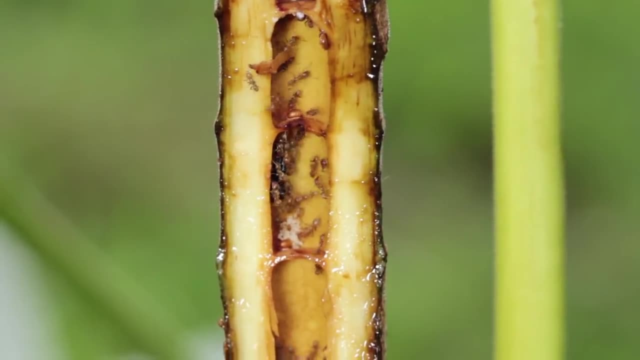 In these regions of high competition amongst plants and animal species for survival, much of this tree's success has been attributed to a special mutualism. Cicropia trees provide a safe, climate-controlled shelter for housing a fierce ant genus known as Azteca. 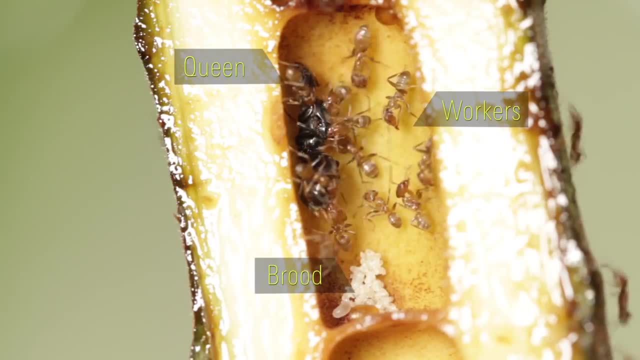 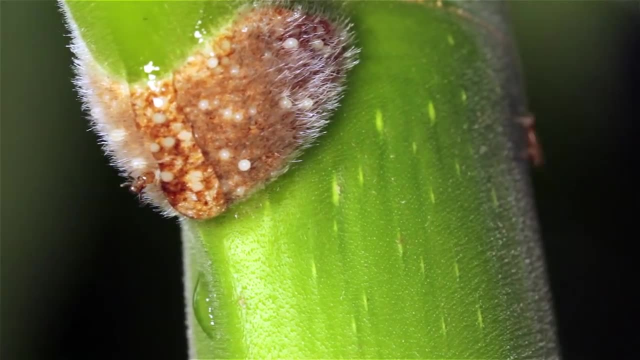 In addition, these trees supply nutrients to their ant colonies through tiny growths called mullerian food-bodies, which are harvested by the ants. They are also known as anemones. In addition, they're also quite pollinating and their habitat is harmful to the plant. 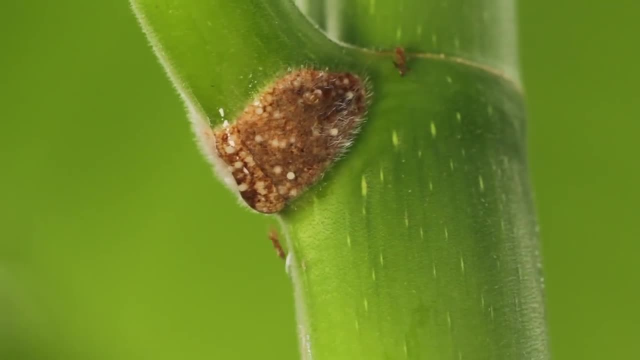 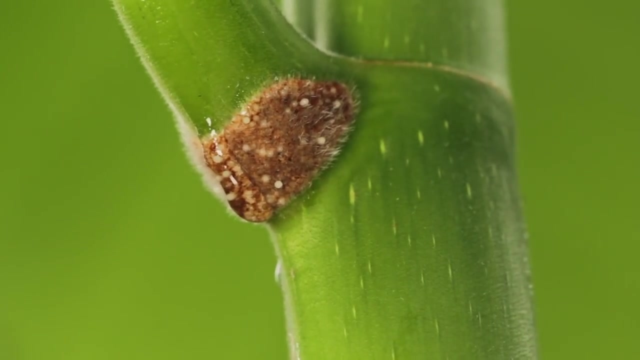 Their very small growth includes the fact that they are not actually a food source-based the plant's population. They are too small for the plant, but are produced exclusively for the nourishment of the Azteca colonies In return for food and shelter. the ants act as the plant's nervous and defense systems. 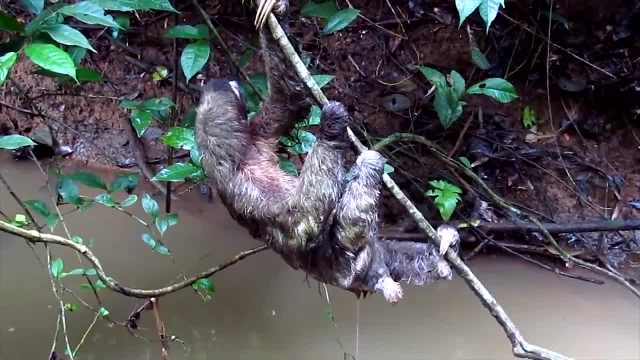 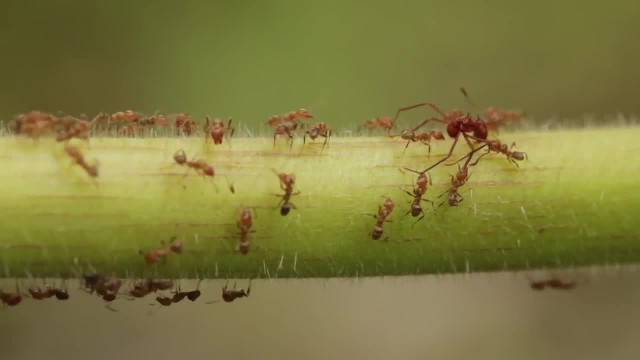 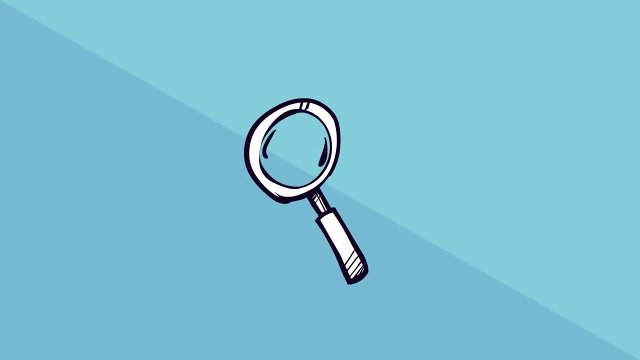 Invasive, destructive elements such as herbivores and leafcutter ants are quickly swarmed, immobilized and removed from the tree. The ants even help the cecropia tree ward off competitive and destructive elements. There are three types of organisms I'd like to look at that have parasitic relationships. 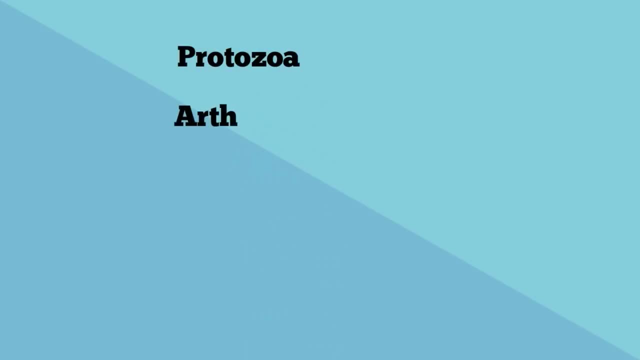 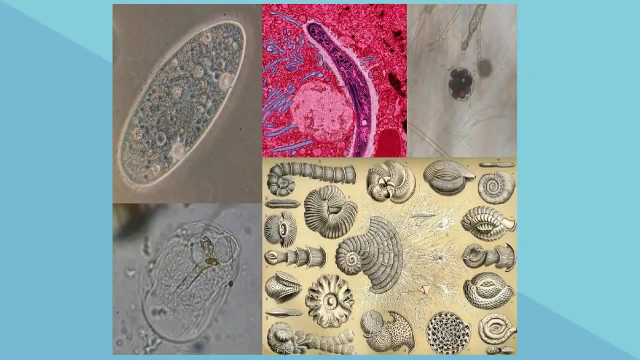 The first is protozoa, the second are arthropods and the third is helminths. Protozoa are single cell organisms that are found in moist areas. Many of them are parasites, like the plasmodium that causes malaria, a worldwide disease. They live in moist areas. 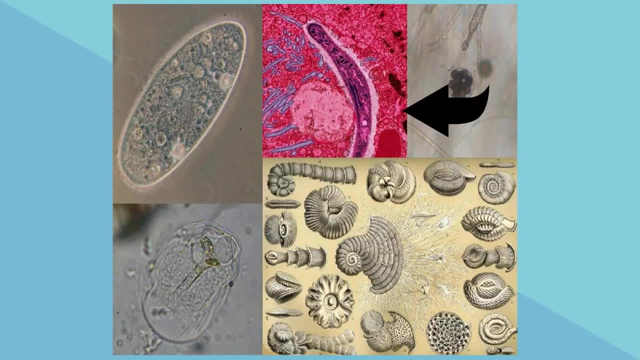 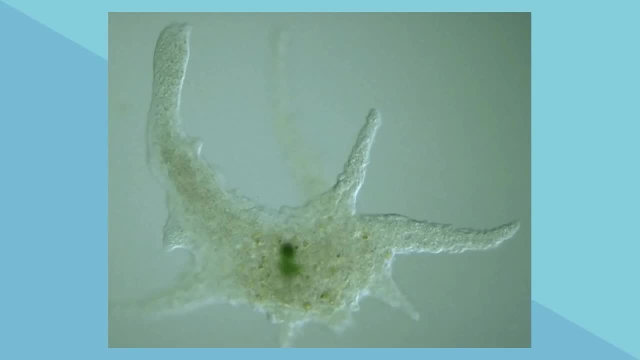 They infect the water. Other animals and humans drink the water and then they become infected. An amoeba is a single cell protozoa and they are sometimes in the news because some of them can be brain eating and result in death, but most just give you an upset stomach. 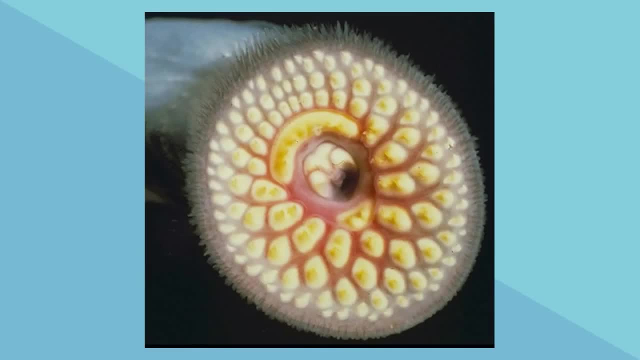 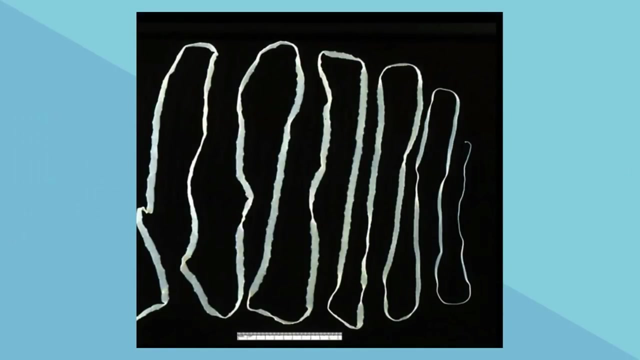 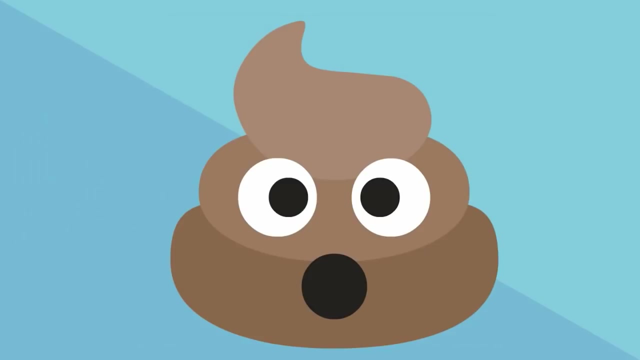 But they are also parasites. The next type of parasite are helminths or worms. There are several types of these. You have a round worm, a fluke or even a tapeworm. The reason why these can be a problem is that many of these worms, such as a round worm or